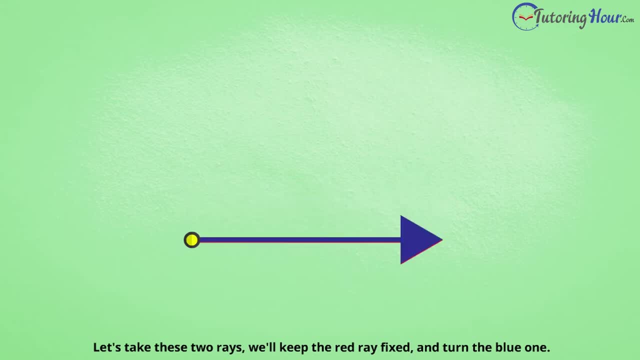 Let's take these two rays. We'll keep the red ray fixed and turn the blue one. As we turn the blue ray about this common point or vertex, you will notice an angle being formed here. We'll draw an arc to represent it like this: The angle is greater than 0 degrees. 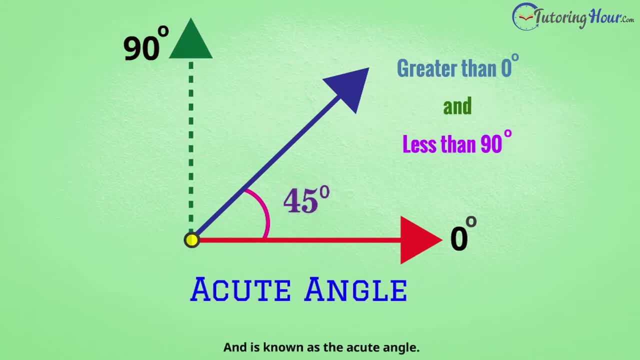 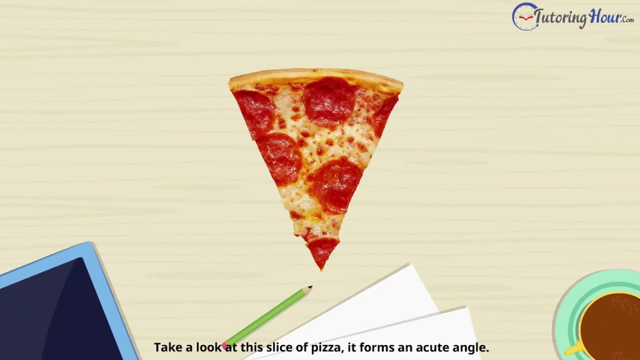 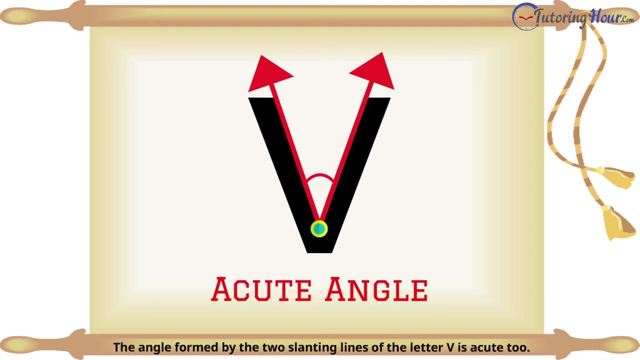 and less than 90 degrees and is known as the acute angle. As we keep rotating, the size of the angle increases. Take a look at this slice of pizza. It forms an acute angle. The angle formed by the two slanting lines of the letter B is acute too. Look at your hand. 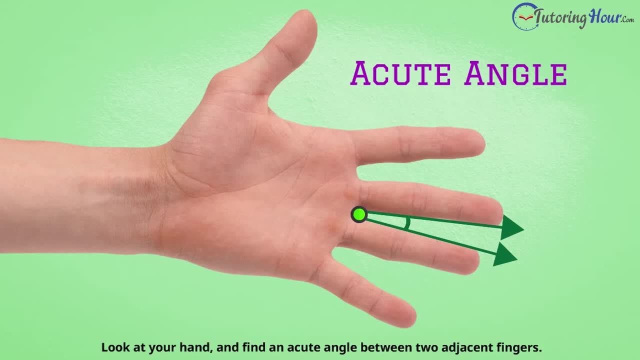 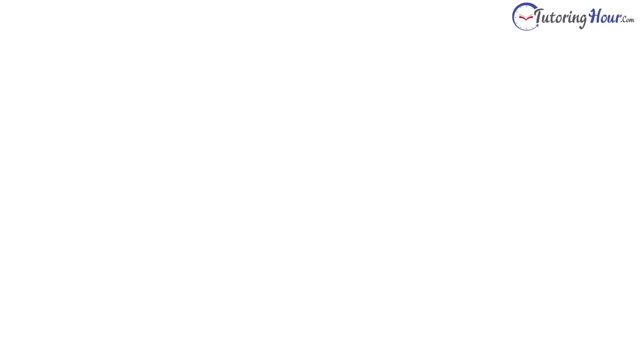 and find an acute angle between two adjacent fingers. Just walk around and you are bound to make a rich list of examples of acute angles. Let's move on to the next type of angle. We'll rotate our blue ray until it points up straight and the angle measures 90 degrees. We have a name for an angle that measures 90 degrees. Do you know? 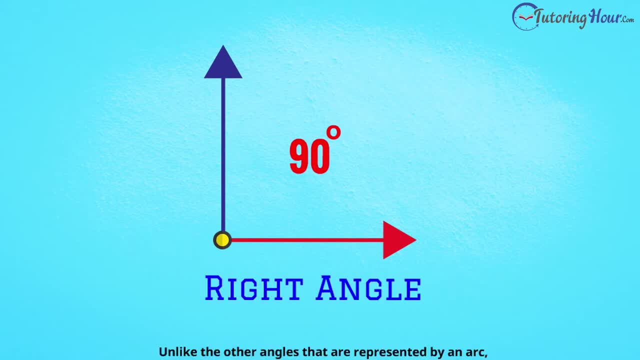 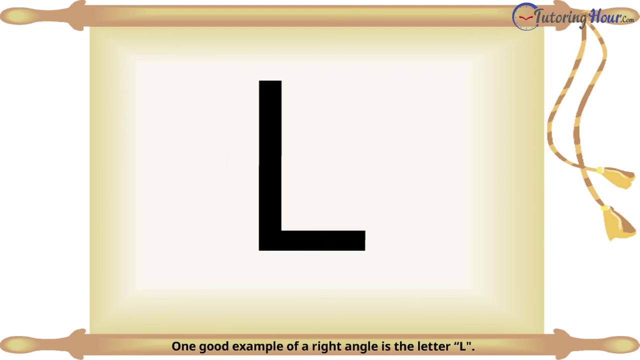 what an angle is. It's called a right angle. Unlike the other angles that are represented by an arc, a right angle is indicated with a little square like this: If you notice carefully, you will find the corners of a room that make a right angle. One good example of a right angle: 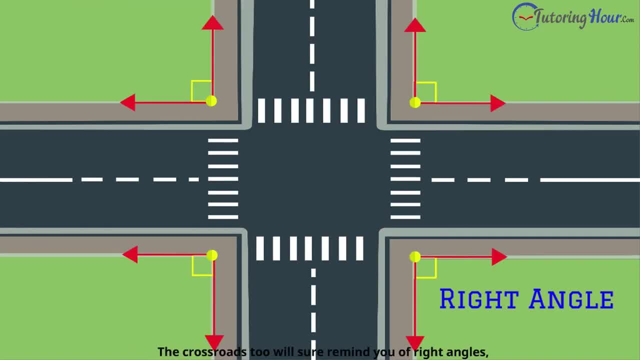 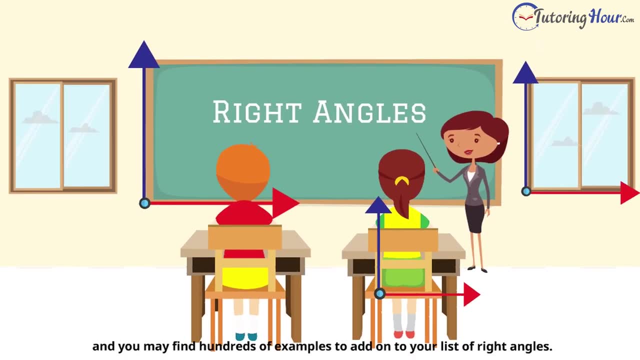 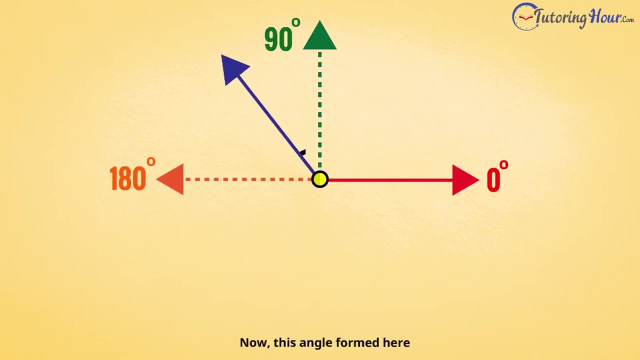 is the letter L. The crossroads, too, will sure remind you of right angles. You just need to look around and you may find hundreds of examples to add on to your list of right angles. Moving on, let's rotate our blue ray past 90 degrees. Now, this angle formed here: 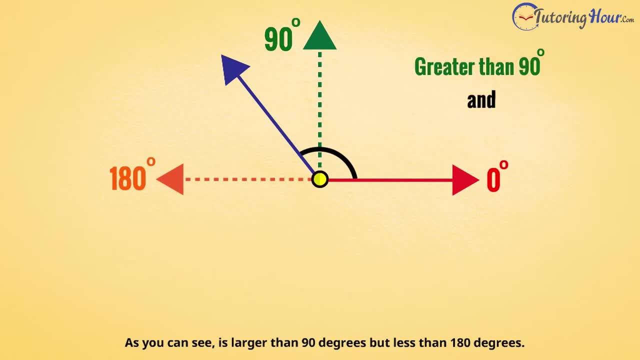 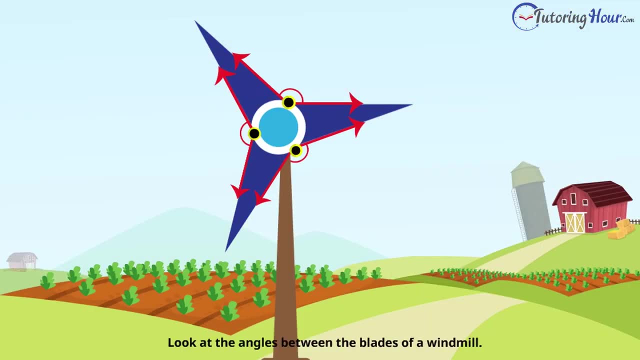 as you can see, is larger than 90 degrees, but less than 180 degrees. This is an obtuse angle. Look at the angles between the blades of a windmill. They lie somewhere between 90 degrees and 180 degrees. Therefore they are obtuse. The letter K has one obtuse angle here. 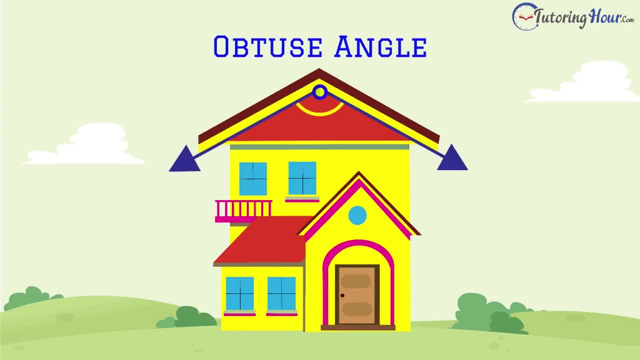 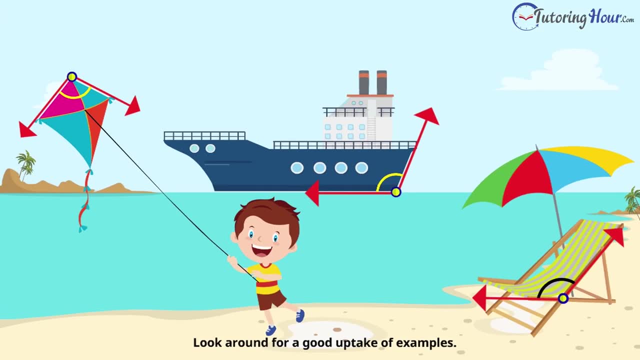 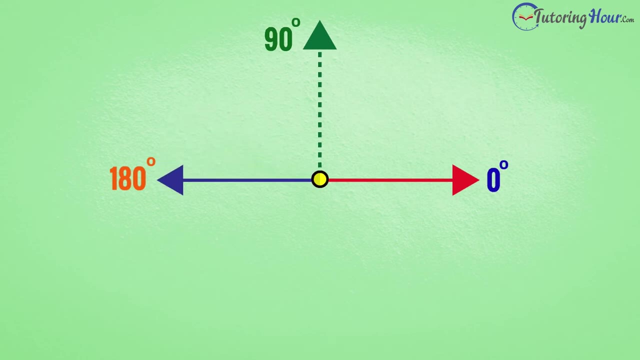 angle in the rooftop of a house. These are just a drop in the ocean of obtuse angles that surrounds you. Look around for a good update of examples. Up next is another important angle. Let's rotate the ray further. Now look at the two rays.